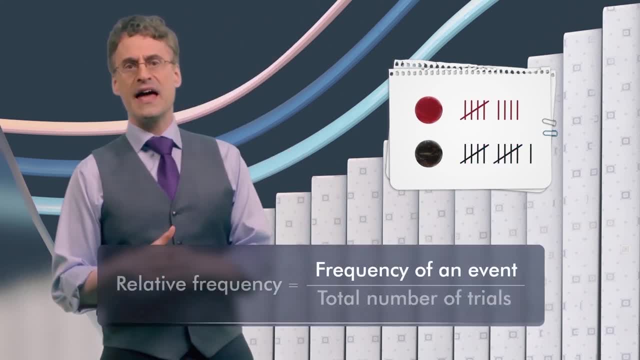 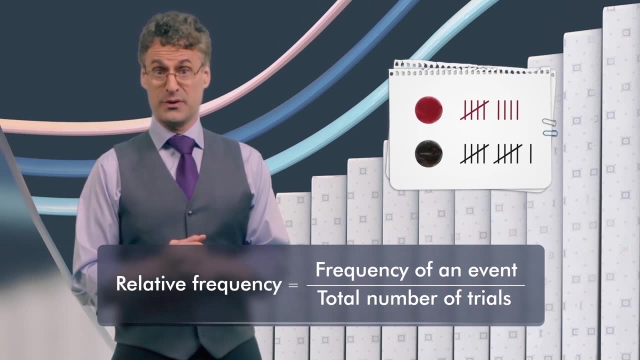 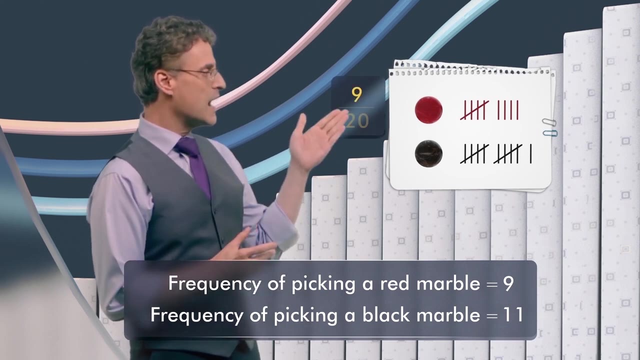 Now, the ratio of the frequency of an event to that of the total number of trials is actually called the relative frequency. Now, with the marbles, the relative frequency of picking a red marble was 9 over 20, or 9 twentieths, because there were a total of 20 trials. 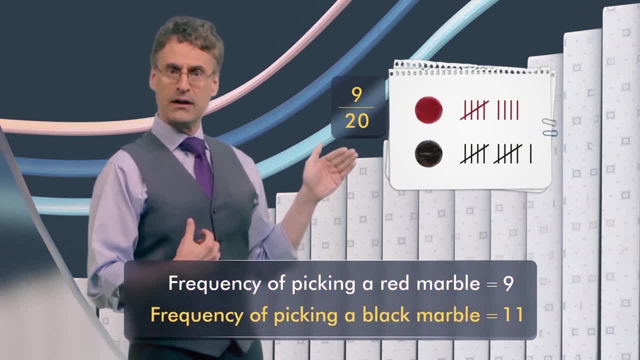 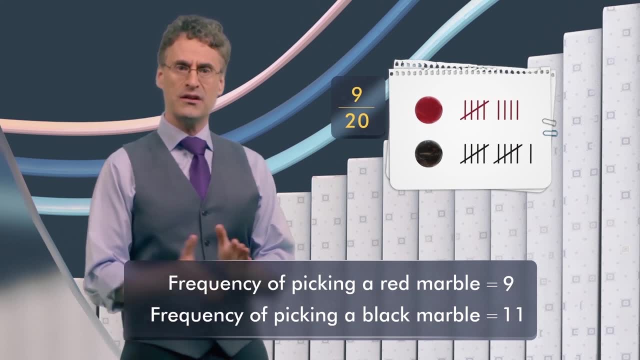 So we saw 9 red and we saw 11 black, which means how many trials were there? We actually add 9 plus 11, and we see there were 20 trials. So there were 20 trials. and so what do I see? 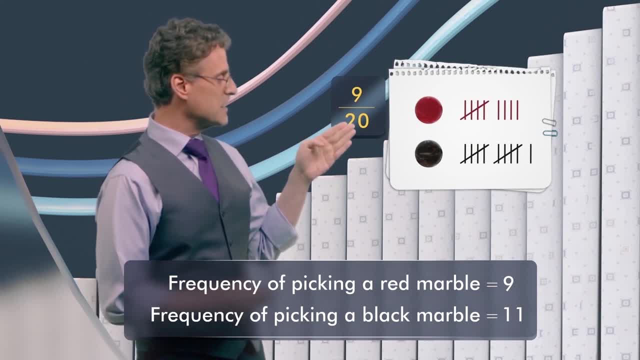 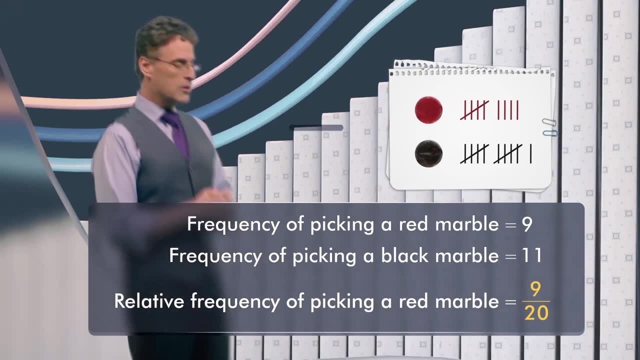 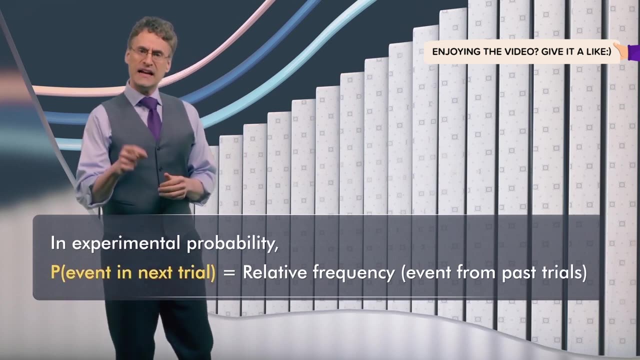 I see that the relative frequency of picking a red was actually 9 twentieths. On the other hand, the relative frequency of picking a black marble was actually 11 twentieths. So in experimental probability for the next trial, the probability of occurrence of an event. 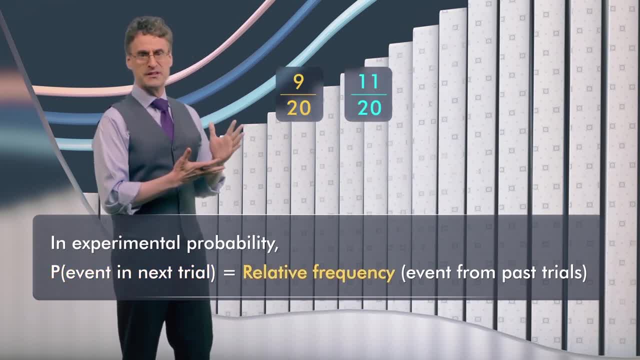 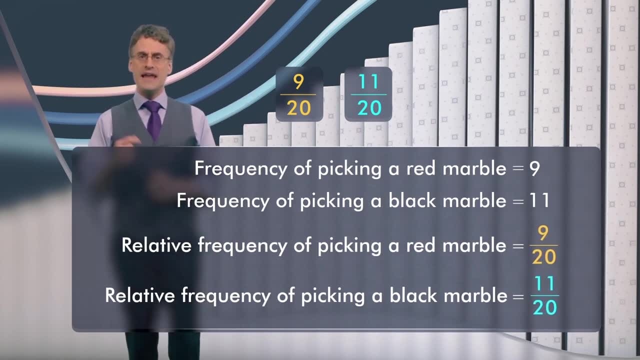 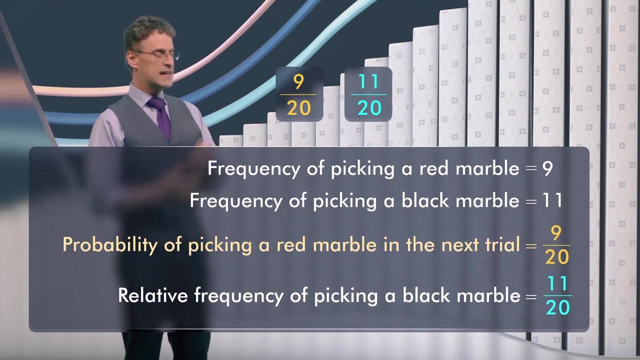 is actually defined to be its relative frequency. So these actually represent probabilities in the case of experimental probabilities. So for the next trial of picking marbles from this particular box, the experimental probability of picking red is actually 9 twentieths, while the experimental probability for picking a black 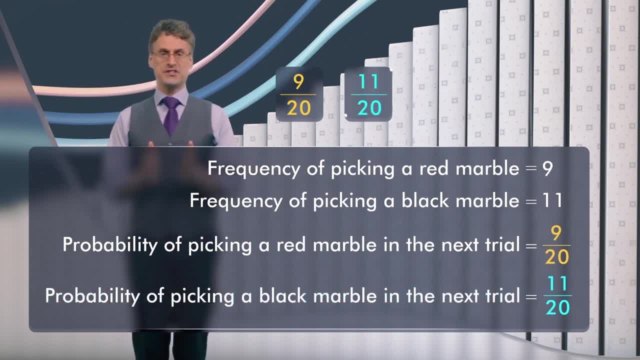 is actually 11 twentieths Interesting. So we get a sense. Now, since 11 twentieths is a little teeny bit bigger than 9 twentieths, then we might guess that it's more likely that the next marble picked is going to be a black rather than a red. 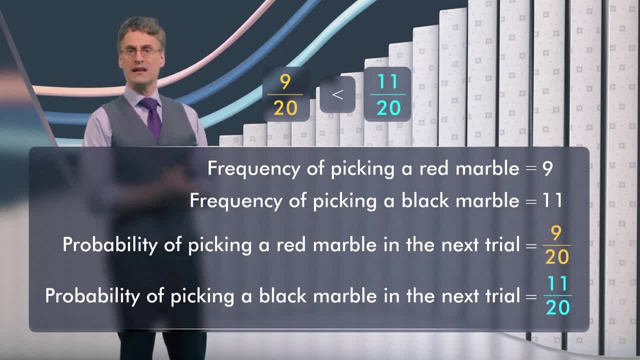 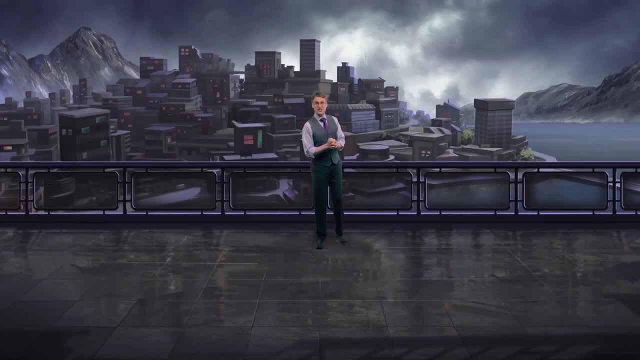 because we've seen black more often than we've seen red, And so in some sense that helps us get a sense of what might be happening in the future. All right, let's take a look at a whole other example. Let's go outside and actually see that there's probability around us everywhere. 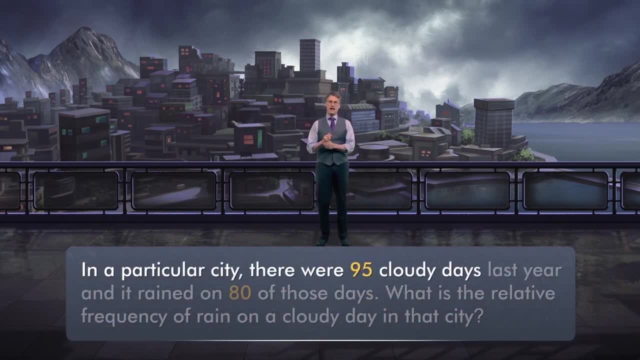 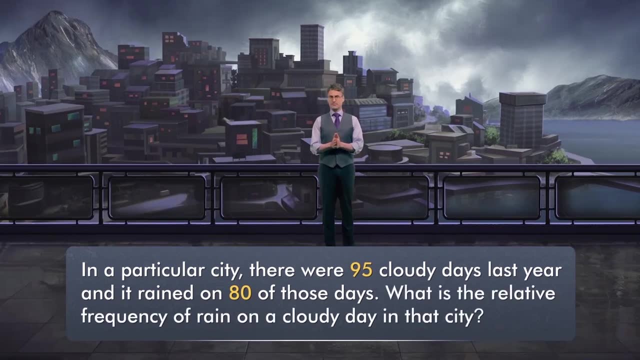 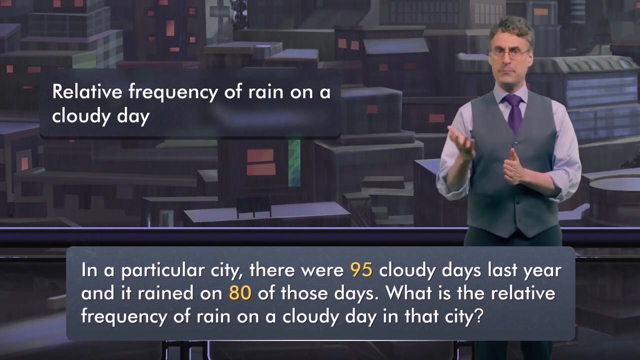 So in a particular city, it turns out that there were 95 cloudy days last year and it rained on 80 of those cloudy days. Well then, the relative frequency of rain on those cloudy days in that particular city was actually going to be 80 divided by 95,. 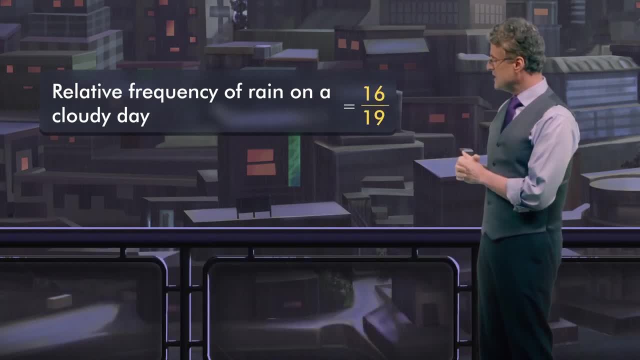 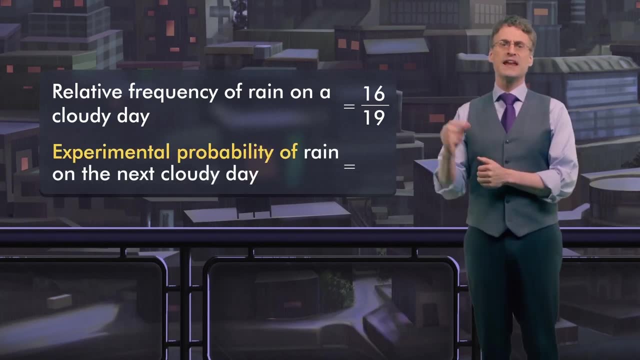 or 80 ninety-fifths, which simplifies to 16 nineteenths. And so, in this case, the experimental probability that it would rain on the next cloudy day in that city is actually 16 nineteenths. And notice that 16 nineteenths is actually very, very close to 19 nineteenths. 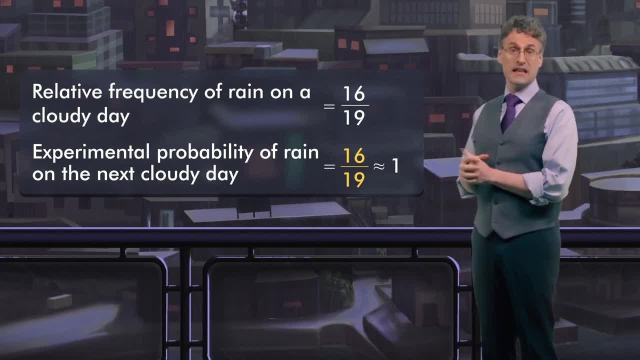 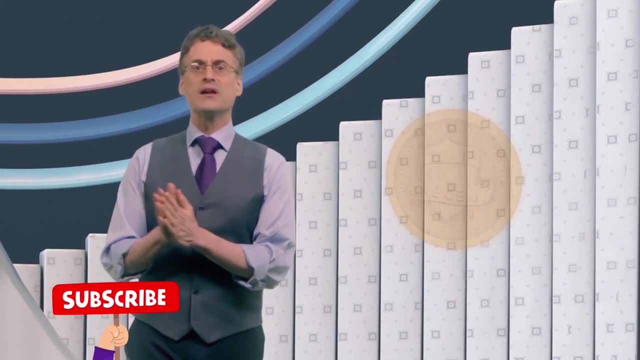 which would actually be 1.. So I'm actually thinking that it's actually very likely that, in fact, on that kind of cloudy day in that city, it's actually going to rain. All right, let's try one last one together. 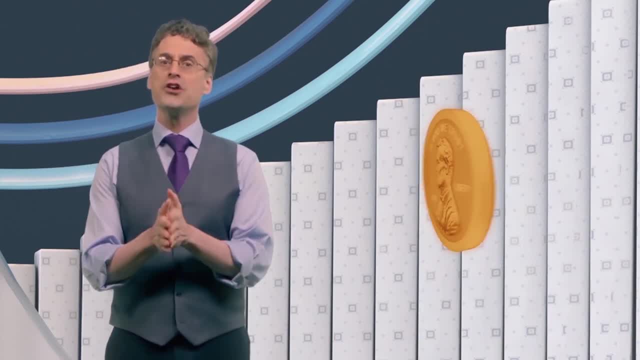 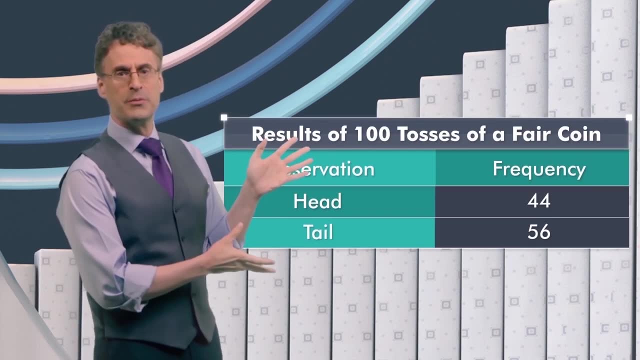 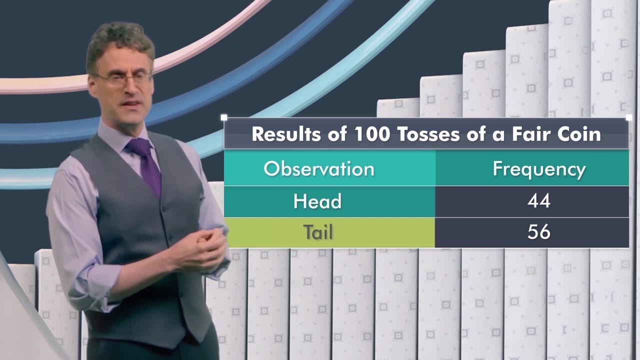 So now imagine, a fair coin is tossed 100 times And what we see from all of those tossings is the following: So here's a little table here where we can actually see that the number of heads observed was 44, and in fact, the number of tails observed was 56. 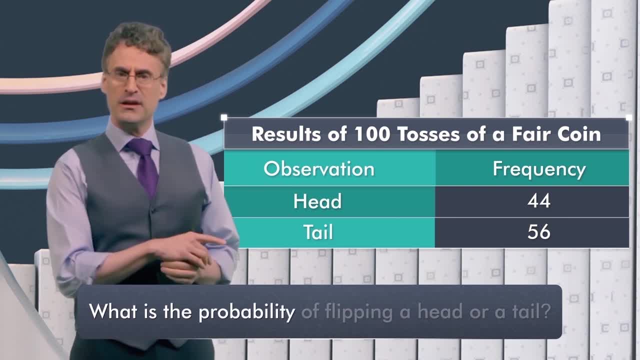 Now, given this data, what is the probability of flipping, let's say, a heads or a tails? Well, again just using this data, we can find the experimental probability by just taking the total number of successes, which, in this case, four heads. 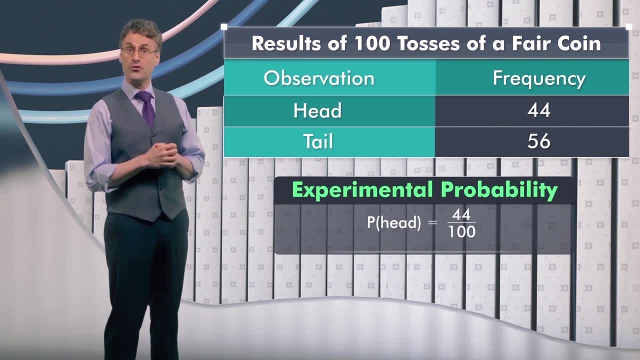 would be 44, and divide it by the total number, which is 100.. And so I'd see a 44 one-hundredths or 0.44.. That's the probability, the experimental probability And the experimental probability for flipping a tails. 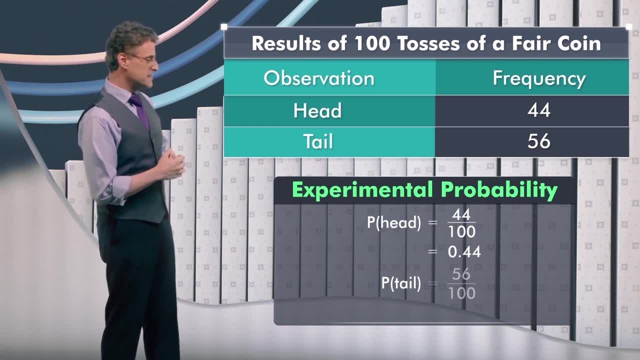 given the data would be the total number of times we've seen tails, which is 56, divided by the total number of flips, total, which is actually 100.. So we see 56 one-hundredths, or 0.56. 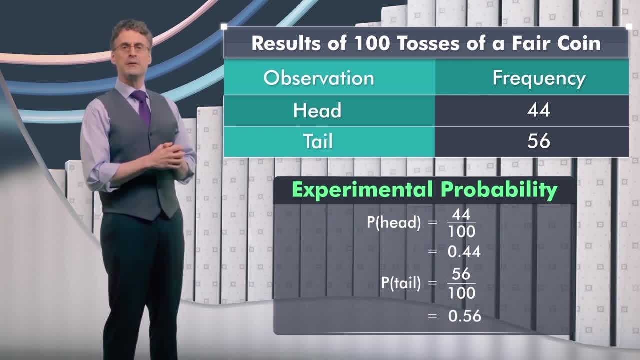 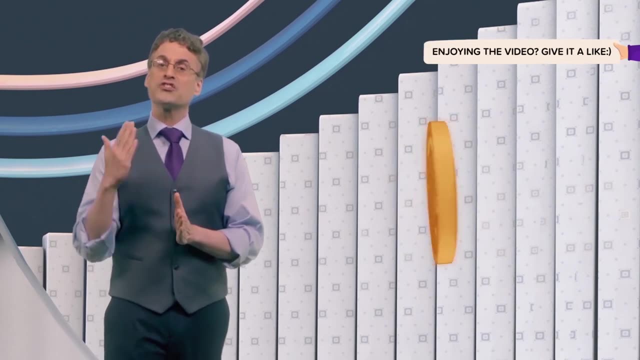 And here you can actually see that there seemed to be a little bit more of seeing tails than we saw heads, And so the computed probabilities in this case, we see, are going to be the experimental ones based on the past data. Now, however, we're told that this particular coin